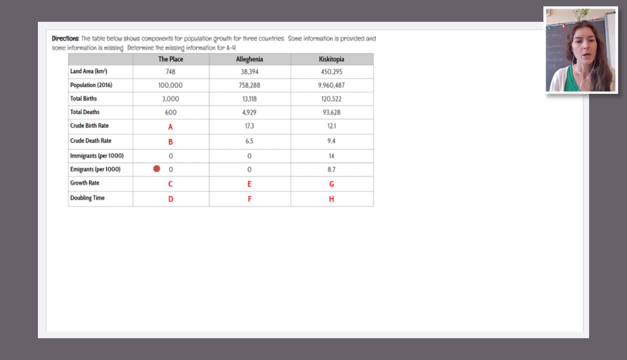 All right. so, first of all, you're given a bunch of information- the population, total population, births and deaths- For some of these crude rates are given, are given or provided for you For the place you have to calculate crude rates. So let's go ahead and get started with that. So remember that crude birth rates or crude death rate is going to be some number of 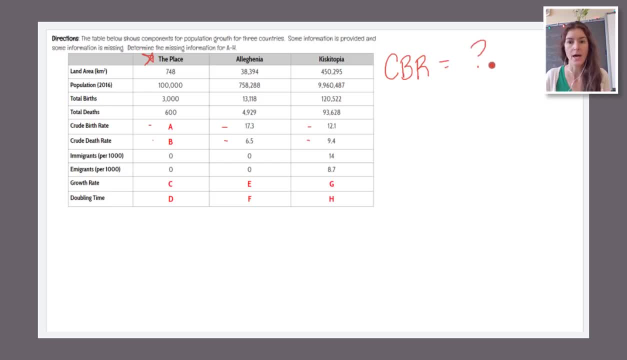 over 1,000. And for the place we don't really know. We don't know what that is, But we are given some information about the total population. So the question is, if there are 3,000 people born in a year out of 100,000 people at the beginning of the year, how many people is that? What's the proportion out of 1,000?? And so this is sort of easy math because you have- you can, excuse me, just eliminate zeros, But I'll go ahead and show you. 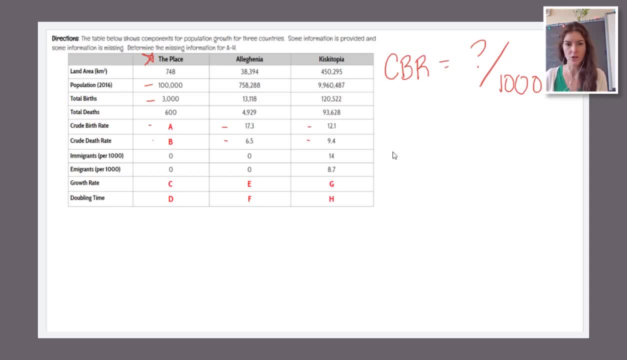 the long way to do this, which is just cross multiplication. So what we do is we go ahead and say that we have 3,000 births out of 100,000 equals x out of 1,000.. So in other words, 3,000 divided by 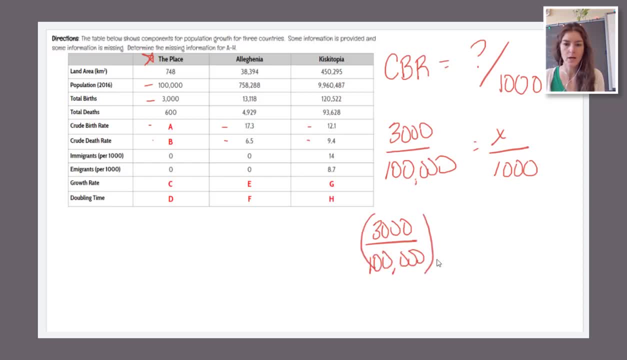 100,000 times 1,000 equals x, And then, solving this, we end up with 30.. So the crude birth rate is 30.. Okay, Let's go ahead and move on to crude birth rates. So the crude birth rate is 30.. Okay, Let's go ahead and move on to crude death rate. 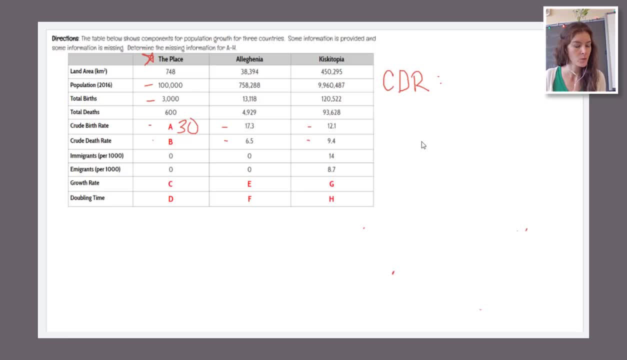 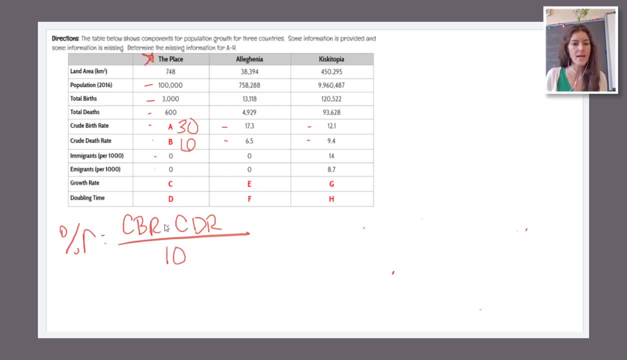 So the crude birth rate is 30. Okay, Let's go ahead and move on to crude death rate. So the crude birth rate is 30.. Okay, Let's go ahead and move on to crude death rate. these are values out of a thousand. When you divide by 10, that will give you your answer. 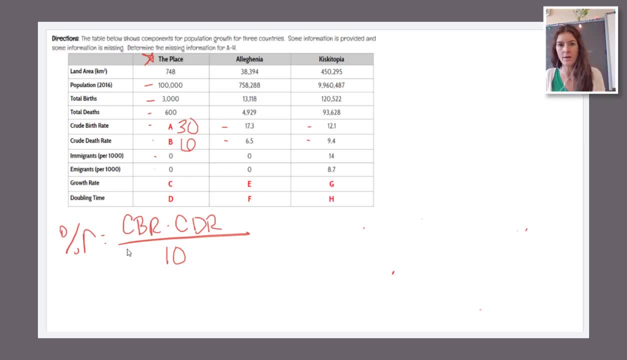 in percent. You don't have to move any decimals. You don't have to multiply times 100.. None of that. This is the formula. Your answer will be in percent. So 30 minus 6 over 10 or 24 over 10 will give you 2.4 percent. That is your answer. 24 divided by 10 is 2.4.. That is the 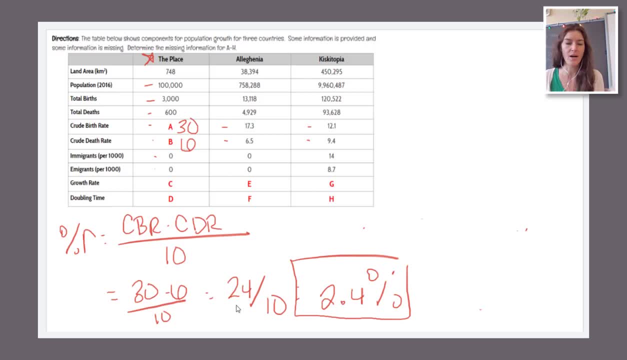 growth rate, That is the number of people that are going to be added every year. 2.4 percent of 100,000 at that rate. Now we can calculate doubling time. So C is 2.4.. Doubling time is 70 over R. This is a very simple way of figuring it out. There's another way to do. 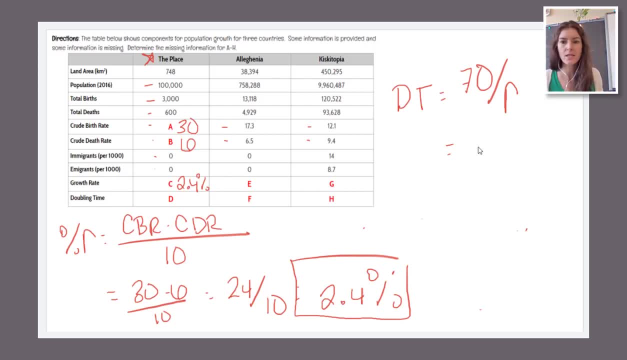 it. This is the easiest thing that you can do: Doubling time: 70 over R. Don't change R, Don't move it out of that format, Don't change the number, Don't multiply, Don't divide this number by anything. This is R, So 2.4. 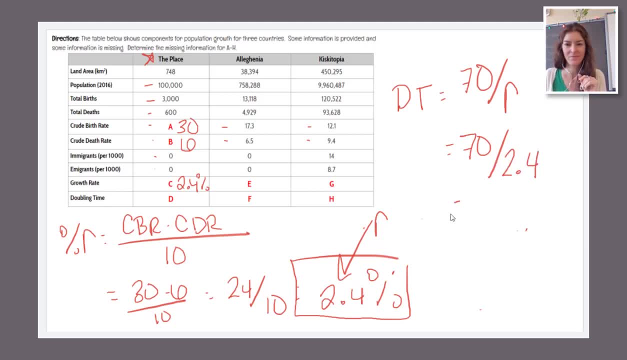 70 divided by 2.4 is 29 years, And again, when you do this, your doubling time will be in years. As long as R is percent, 29 years. Okay, Let's move on to this fake place, Alleghenia. So, Alleghenia, you're actually given crude rates. 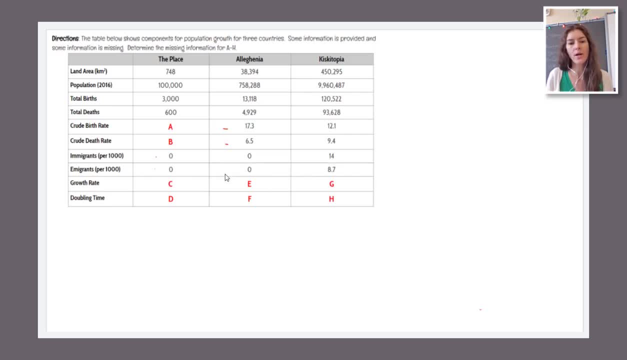 And so that makes it pretty easy, And you also don't have immigrants or emigrants, So we're saving a step from the previous problem. You do have decimal points in this particular one, though, But let's go ahead and calculate E growth rate. So rate is crude birth rate. 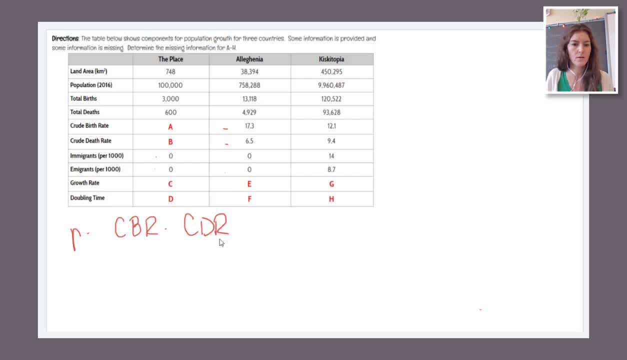 Minus crude death rates Over 10. Or 17.3 minus 6.5. Divided by 10. Okay, Okay, Okay. And then we get 10.8 over 10. And so our answer is 1.08%. 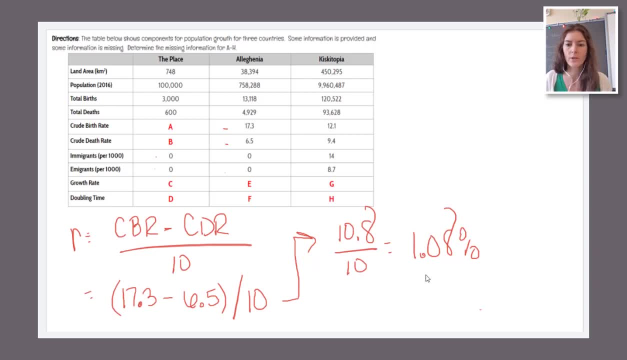 Now the directions tell you to round to the nearest tenths place for growth rates, And so your answer that you would type in is just 1.1.. And I told you to leave out units and everything. So you would leave out that percent, but your answer would be 1.1%. 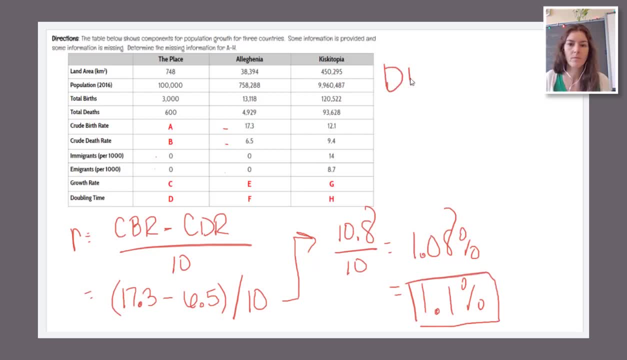 Okay, great, And then doubling time. It's really simple: 70 over R. Again, don't change R. Leave it 70 over 1.1.. Now you could do 70 over 1.08.. And then you wouldn't have to worry about you know incorrect. 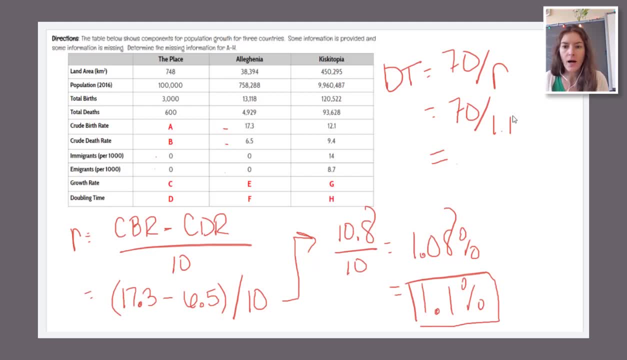 Decimal placement. But I did accept a variety of answers. So let's just say 1.08.. When we divide that, we get 64.8.. And your answer is: years Now I wasn't sure if people would divide by 1.1 or 1.08.. 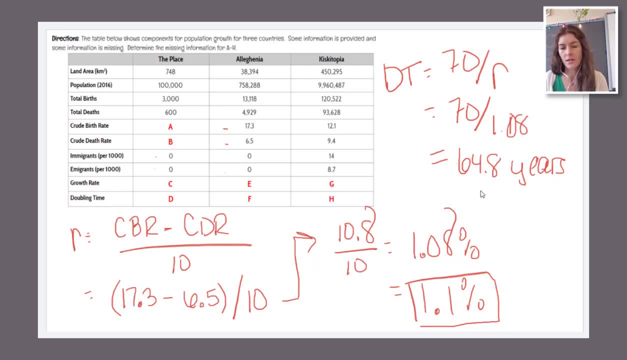 So I did accept 63,, 64, or 65.. The question asks you to round to the nearest whole number, So 65.. 65 is the best answer there. All right, Let's move on to Qiskitopia. 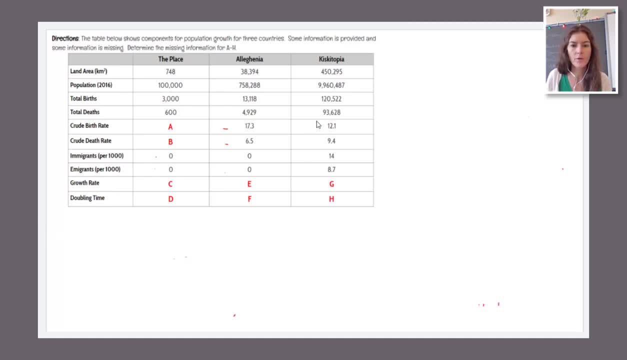 So for this one you had crude birth, crude death, and you had immigrants and emigrants, And so you have inputs and you have outputs for a couple of different reasons here, And so you always are going- growth rate is always no matter what- going to be inputs minus outs. 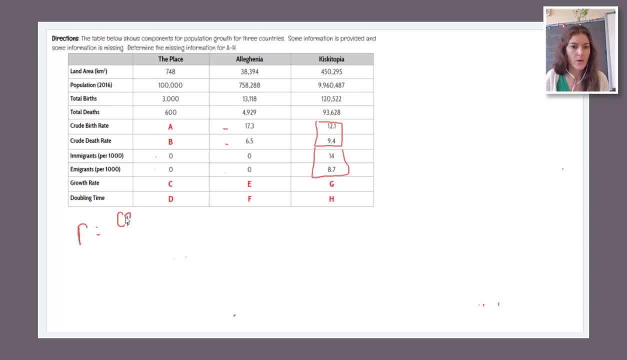 So let's go ahead and add together our inputs, So crude birth rate plus the other input would be from immigrants, Okay, Inputs minus outputs, And then our outputs would be crude death rate minus the immigrant rate, And then, since all those numbers are out of 1,000,. 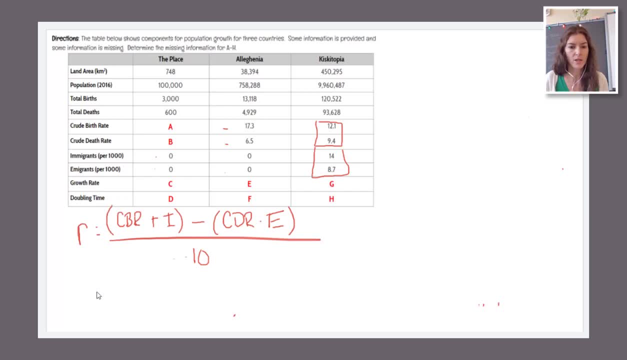 when we divide by 10, that's going to give me growth rate in percent, and then when I substitute my values in here, it's 12.1 plus immigrants per 1000 is 14 minus 9.4. adding together my outputs plus 8.7 over 10 and then calculating: 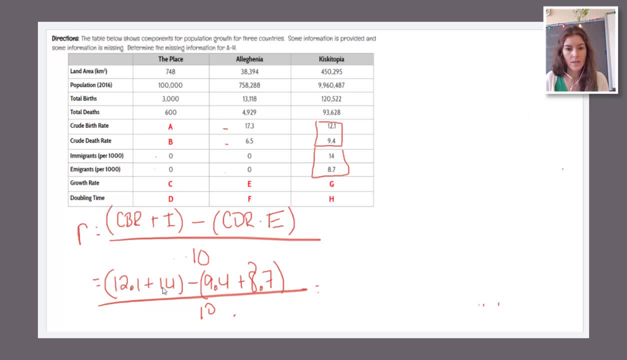 this I end up with- and it's nice if you take it step by step, because that way you can check your answers- you end up with 26.1, let's see. you end up with 26.1. let's see, yeah, 26.1 minus 18.1 over 10, or 8 over 10, which is just 0.8, 8 tenths of a.